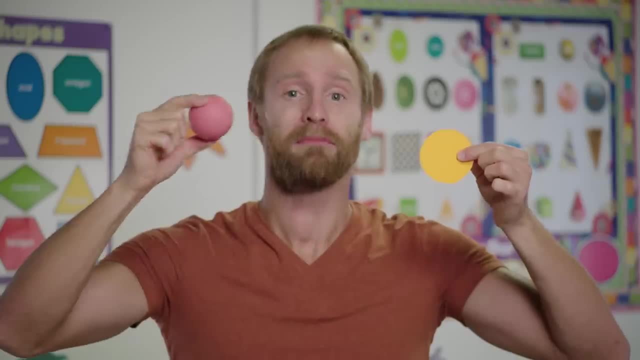 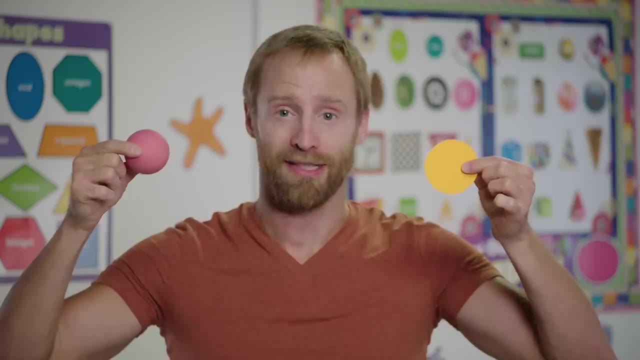 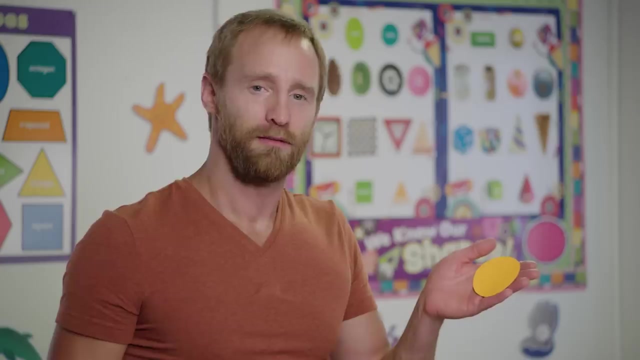 This sphere is still pretty puffy and full, It must be a 3D shape. We can further experiment with the flatness of a shape by doing the clapping test. Are you ready for that, Bob? You bet. Remember, if the shape is flat, it's a 2D shape and you should still be able to clap. 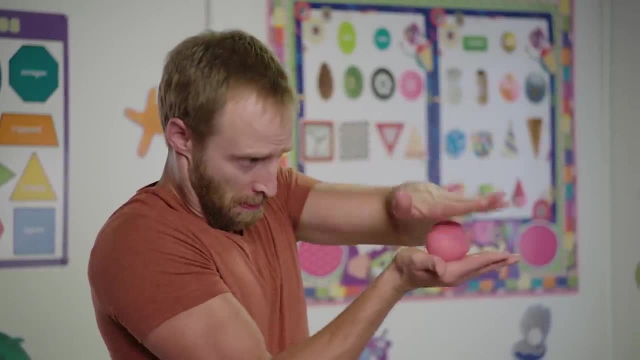 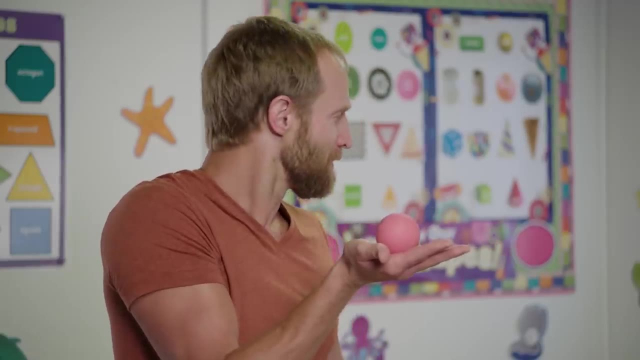 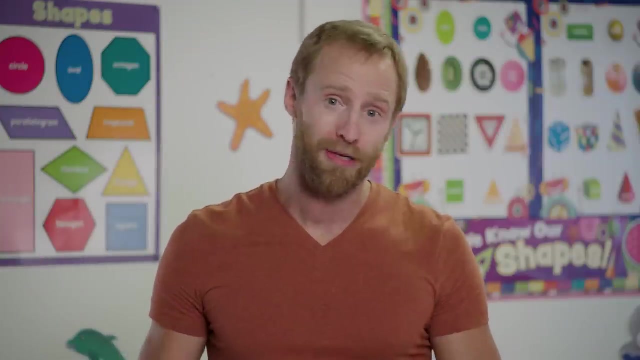 Now let's try the 3D shape. Oh no, The 3D shape is too puffy, It sticks out too much. I can't clap- Sorry, Bob, The music's over. Oh, If you're still not sure if a shape is 2D or 3D, there is one more way to test. 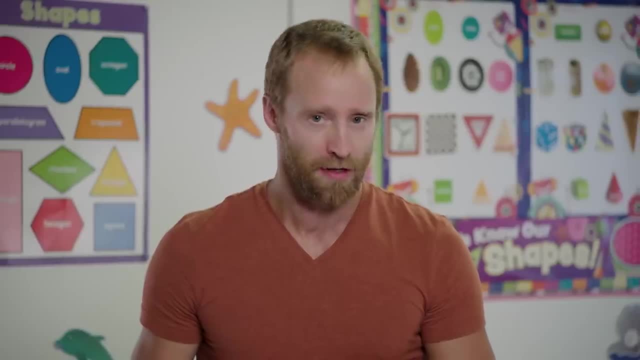 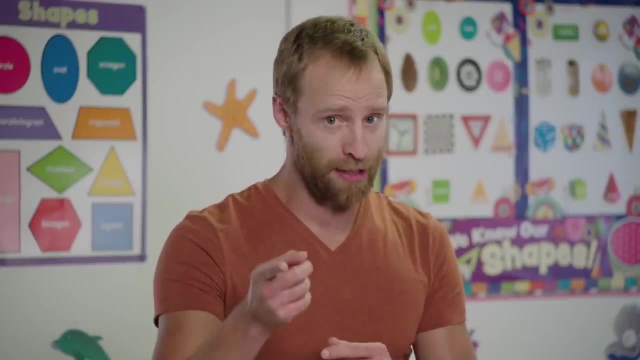 but leave this one to me Because it's kind of dangerous. all right, It's called the sit test. Here's what's going to happen: Bob's going to put a shape behind me and I'm going to sit down. If it's a 3D shape, I should be able to sit. 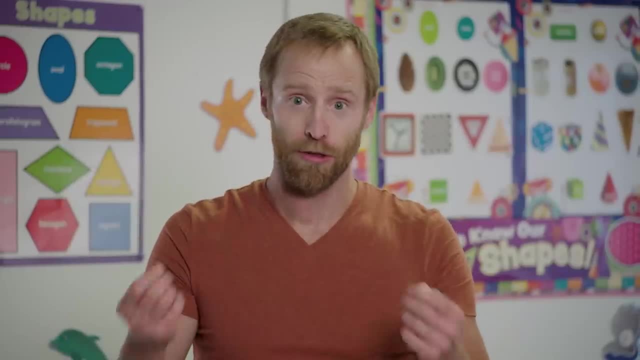 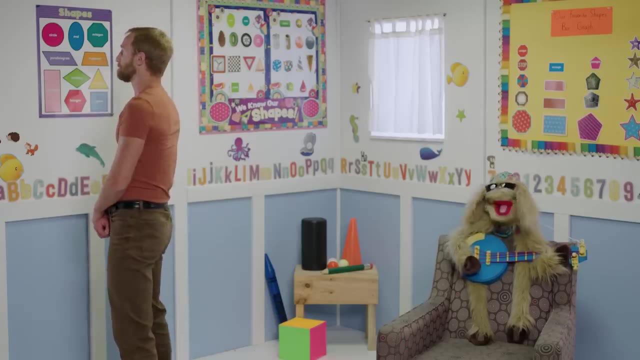 because 3D shapes are full and they stick out, But if it's a 2D shape I might be in some trouble. Are you ready, Bob? Give me the first shape. Okay, Mr B, Here we go, Give me the first shape. 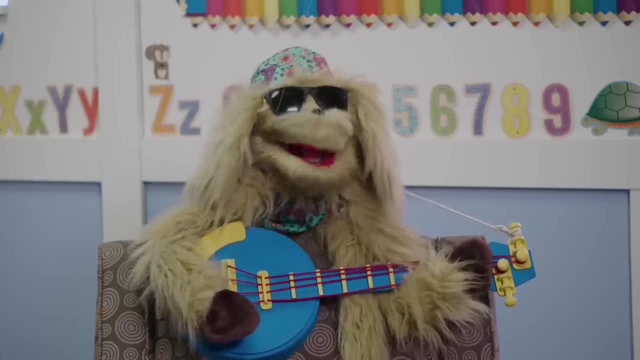 Okay, Mr B, Here we go. Give me the first shape, Give me the first shape. Give me the first shape. Okay, Mr B, Here's the 3D shape. Give me the first shape. Mr B, here comes a sphere. 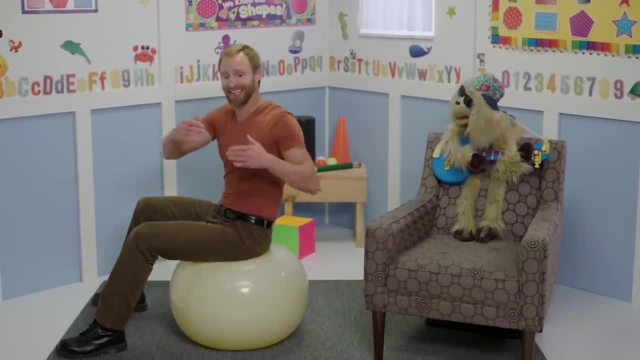 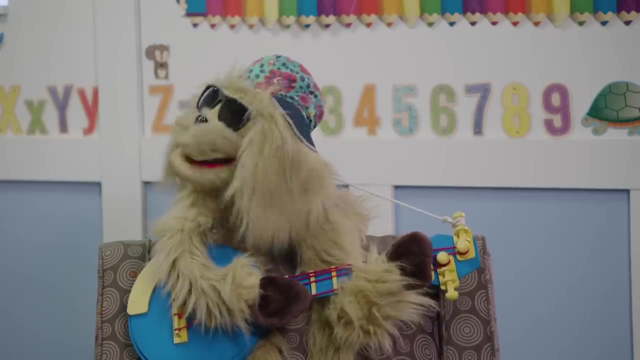 Oh, wow. A sphere must be a 3-D shape. It sticks out three ways and keeps me off the ground. Thanks, Bob. Good job, Mr B. How about another one? Yep, Bob, I'm ready, Give me the next shape. 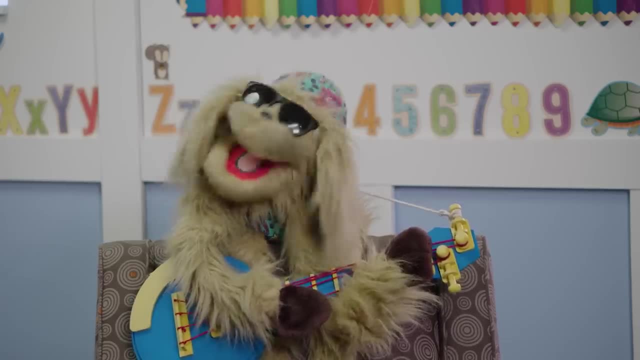 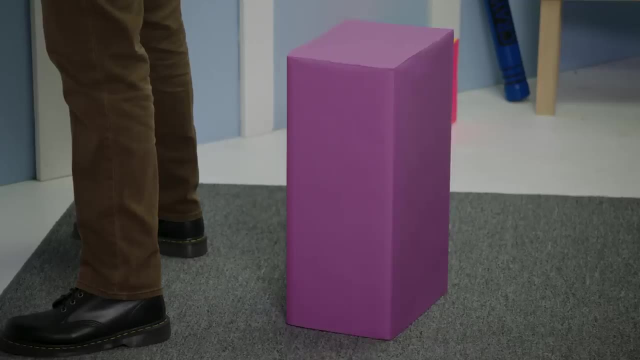 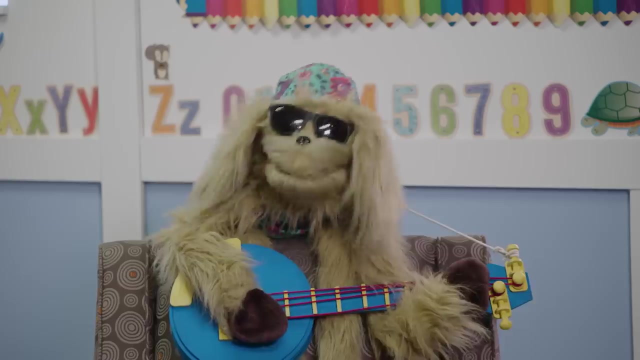 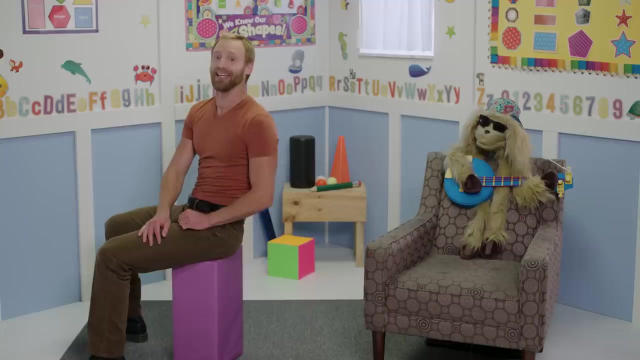 Okay, Mr B, how about a rectangular prism? Whoa, Rectangular prism must be a 3-D shape, because it kept me off the ground, Bob. That's crazy. It goes side to side, front to back and up and down to keep me from falling. 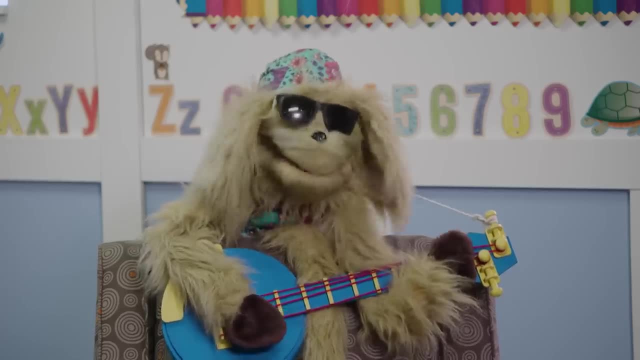 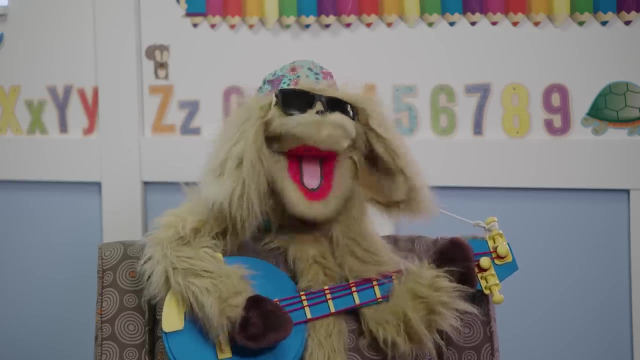 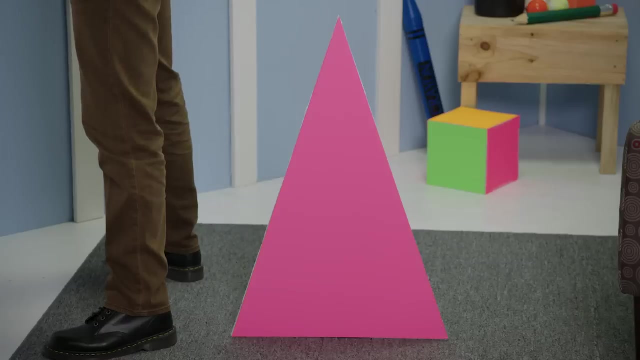 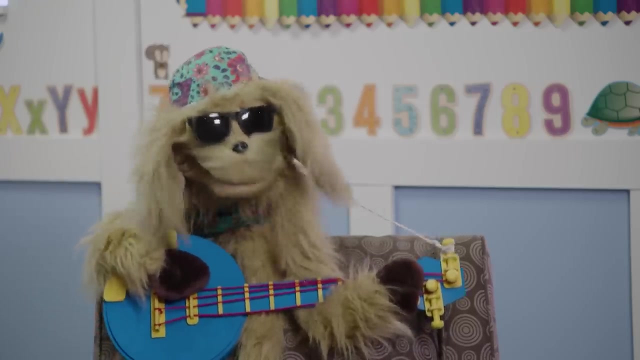 Pretty cool guys. Okay, Mr B, time for the last shape. I'm ready. when you are, Bob, Give me the last shape. Okay, kids, let's try a triangle. Oh no, That definitely wasn't a 3-D shape, Mr B.